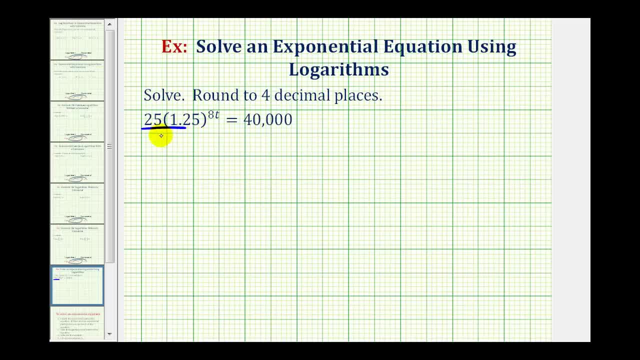 which means the first step is to divide both sides by 25.. On the left side, 25 divided by 25 simplifies to one. so we have 1.25. raised to the power of eight, t equals 40,000. divided by 25 is equal to 1,600.. 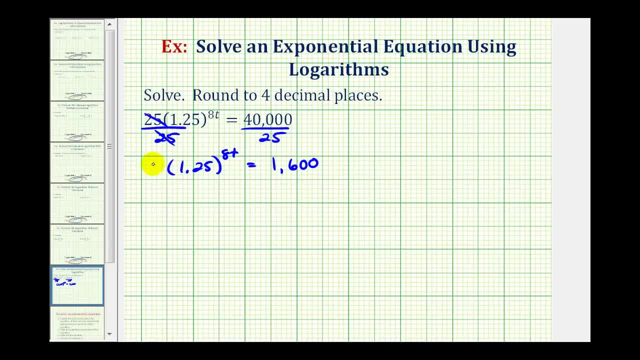 Now to solve for t. we want to move eight t out of the position of the exponent. To do this we can take the common log or natural log of both sides of the equation. We need to use common log or natural log because we are going to have to use the calculator. 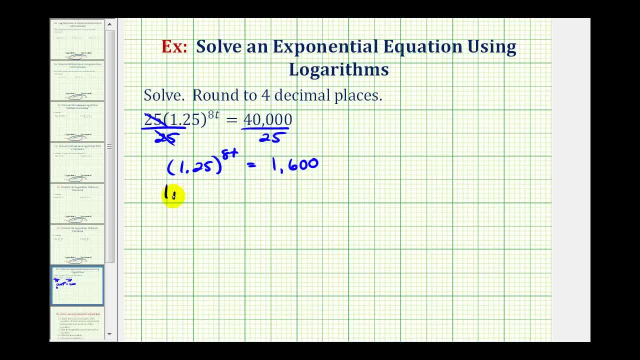 Let's go ahead and take the natural log of both sides of the equation. So we'd have natural log of 1.25 raised to the power of eight. t equals natural log of 1,600.. Now, looking at the left side, we can use the power property of logarithms. 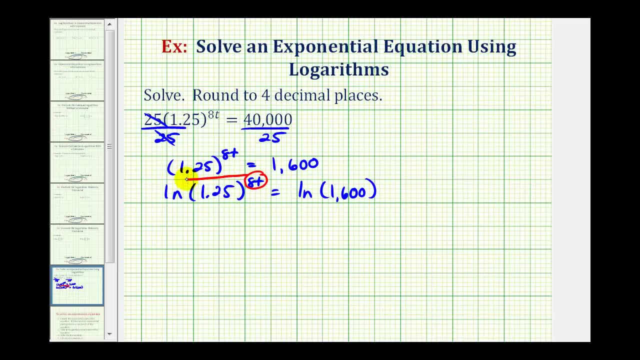 to take the exponent of eight t and move it to the front of the logarithm, so we have eight t times natural log 1.25.. So again we'd have eight t times natural log. 1.25 equals natural log 1.25. 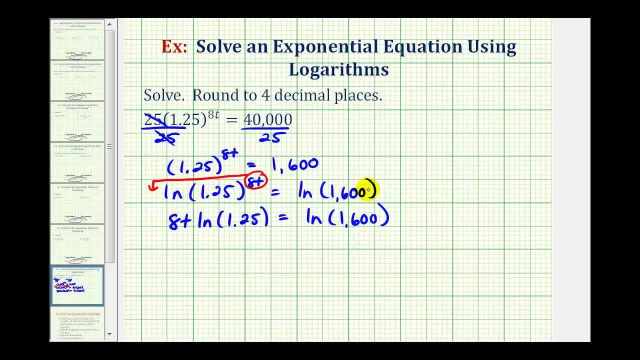 So again we can use the common log or natural log of 1,600.. Now, remember, our goal is to solve for t. so eight and natural log 1.25 are attached to t by multiplication, which means now we'll divide both sides. 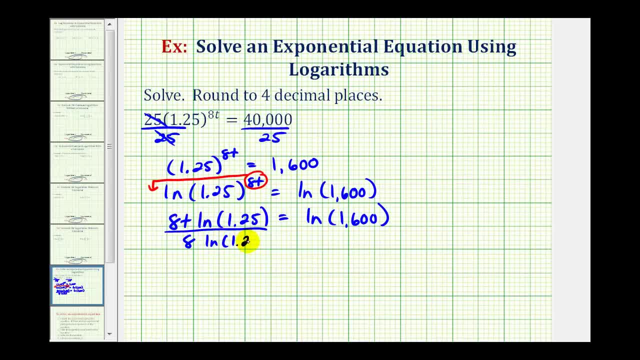 by eight: natural log 1.25.. And of course we'll do this on both sides. Looking at the left side, eight divided by eight is equal to one: Natural log 1.25 divided by natural log 1.25 simplifies to one. so we're left with t. 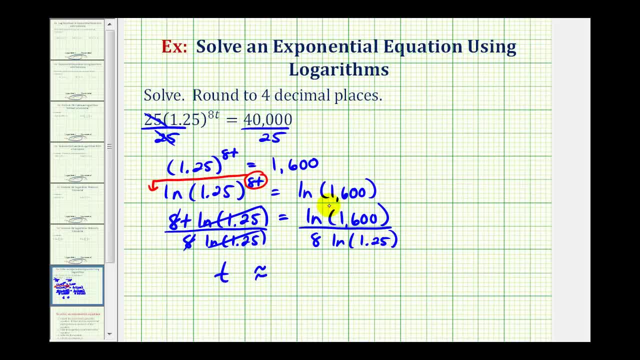 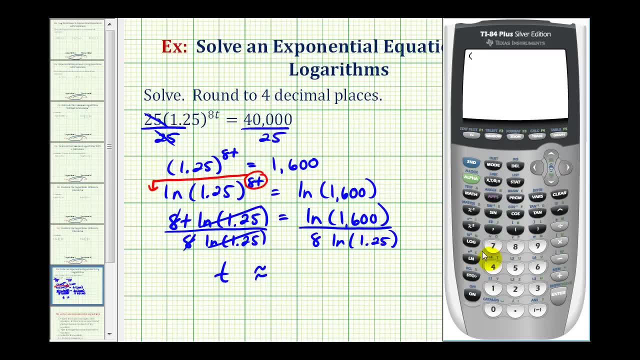 And now we'll have to go to the calculator to get a decimal approximation for this quotient here. So I'll put the numerator in a set of parentheses as well as the denominator. So the numerator is going to be natural log 1,600..